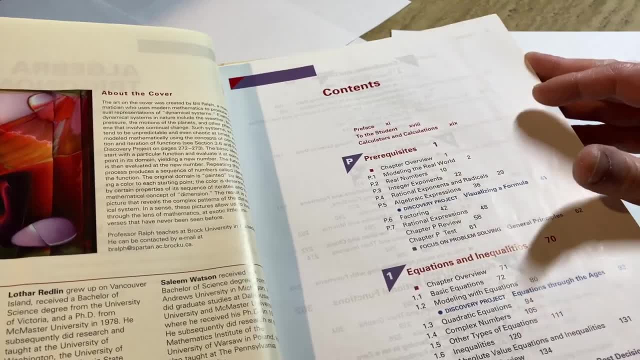 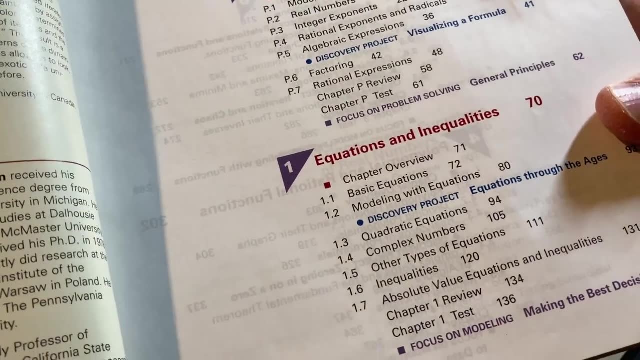 algebra and trigonometry. So it's also used for courses such as precalculus. So it starts with equations and inequalities. So quadratic equations, complex numbers, inequalities. So you have a lot of basic algebra. Let's jump to the trig. 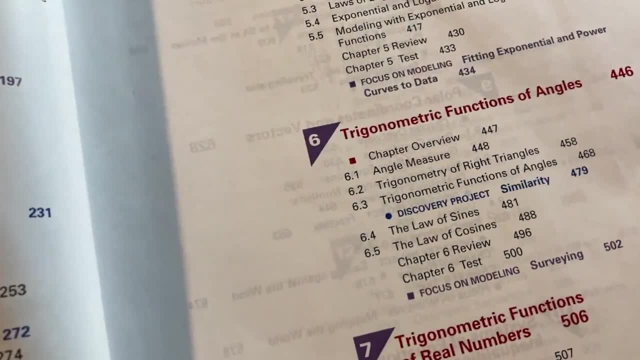 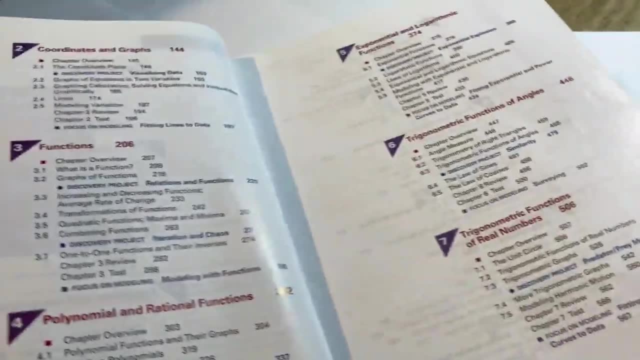 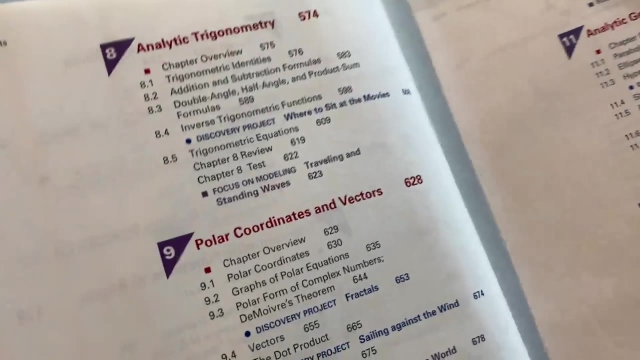 So here's where the trig starts: Trig functions of angles, Trig functions of real numbers. That's where it talks about the unit circle. Trig is tough because you really have to learn the first stuff. you learn, Like when you first start the class. the stuff you learn at the beginning is: 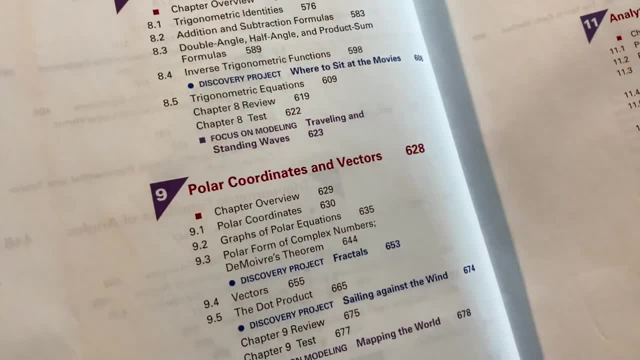 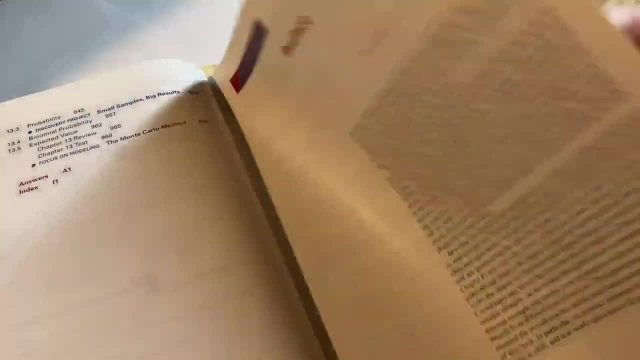 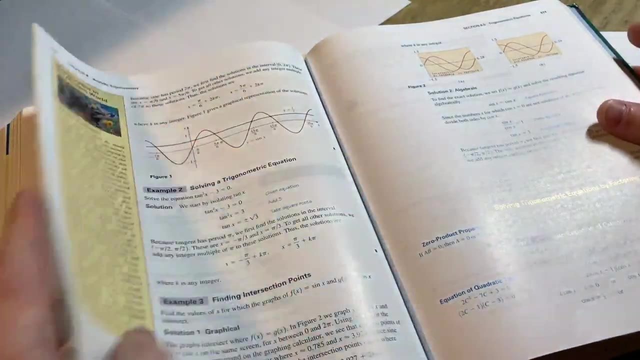 really important Analytic trigonometry, polar coordinates and vectors, And that would be it So great for learning trig. Let me just show you some of the examples so you can see what they look like. Trigonometric equations: this is actually one of the hardest. 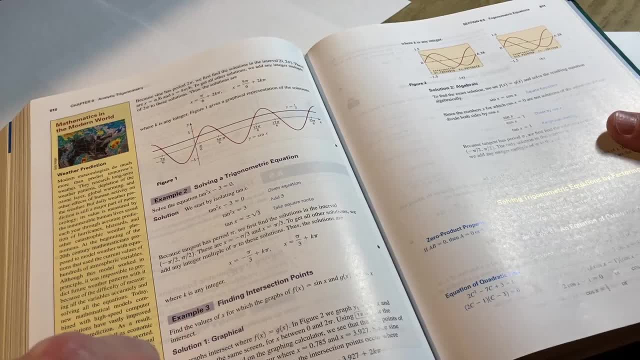 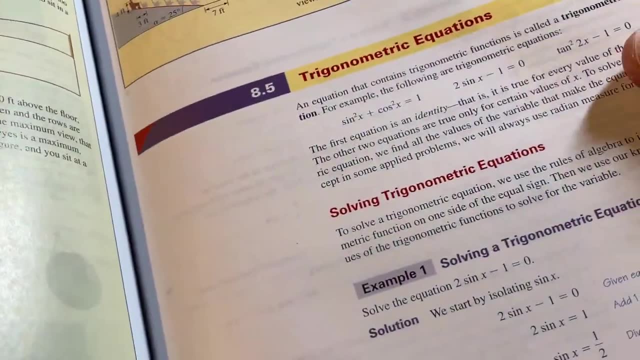 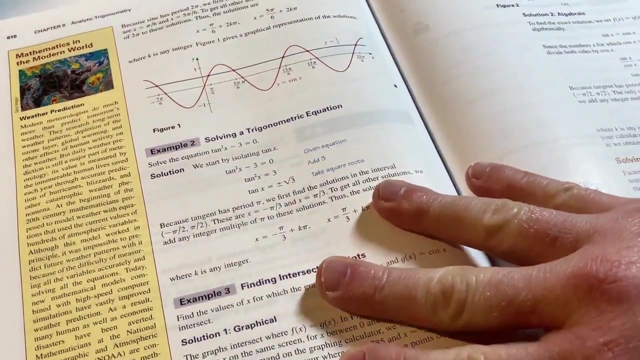 things for people who take trig. It's solving trig equations. So you see, the book does have a lot of examples. You have one example here which is pretty easy: Two sine x minus one equals zero. That's pretty easy. And the page and they solve all this. So they find out, he finds all the solution. 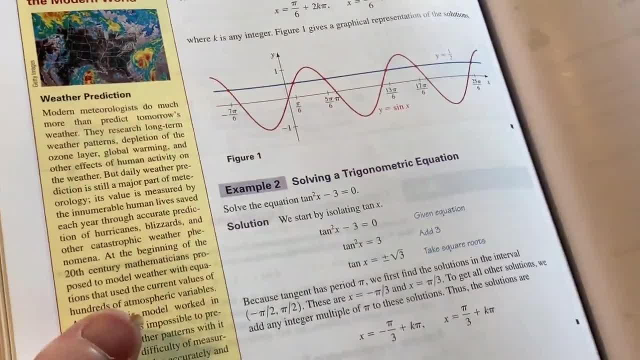 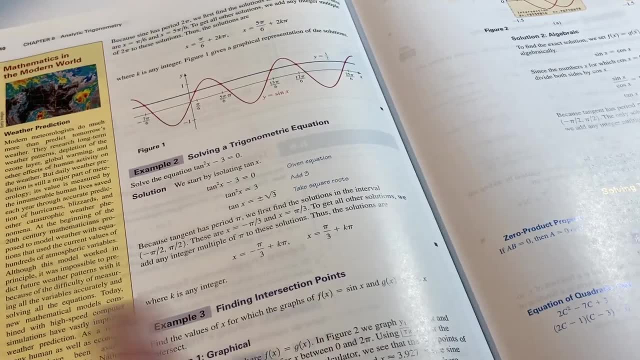 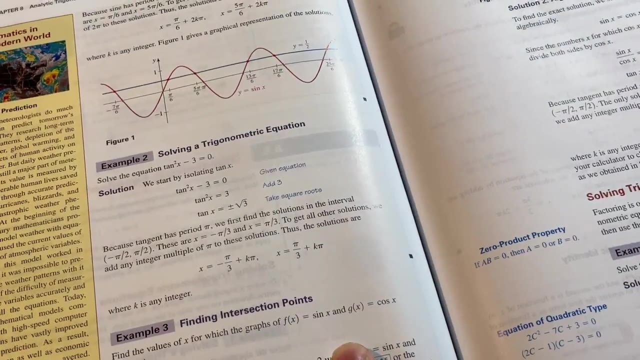 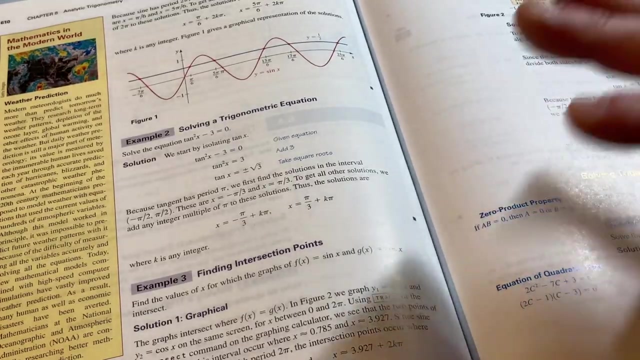 right, they find all of them. that's cool. then here's one with tangent squared. then something about finding intersection points. they set sine equal to cosine. that's interesting. i remember having to do that uh in an unrelated problem and i didn't know how to do it. i remember it was a. it was a complex variables class, so way more advanced uh than 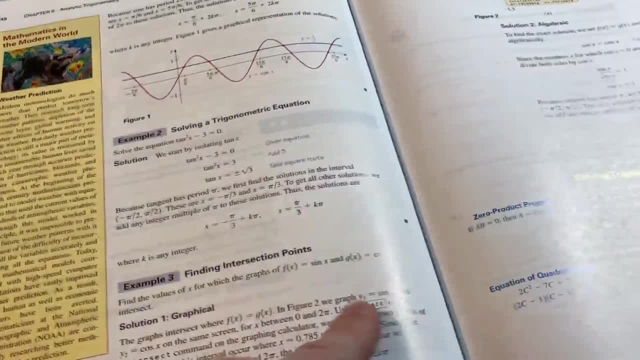 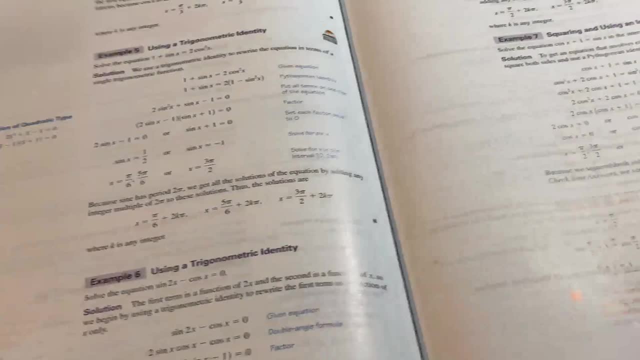 trig and i didn't know how to do that and that's what held me up in the problem. so really, really good that this example is in the book. i don't know brings back some memories of being stuck, but you learn right, it's all about learning lots of examples. 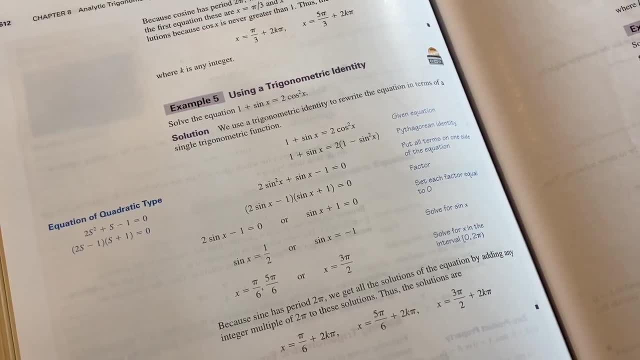 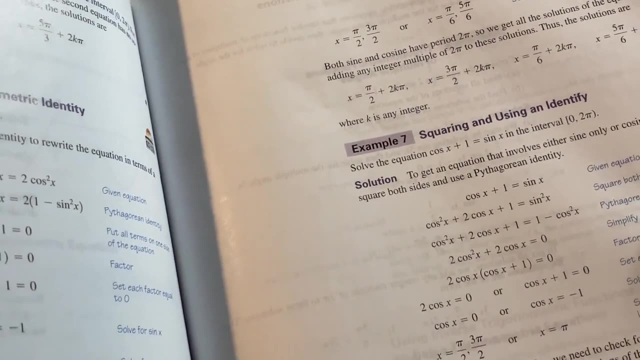 here's one where you have to use a trig identity. one plus sine x equals two cosine squared x. and here's one where you square it and use an identity. wow, so lots of examples. yeah, wonderful book. so that's one example of how to do that, and i'm going to show you how to do that in a minute. 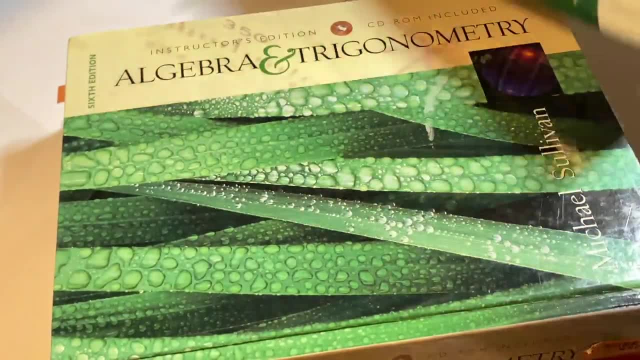 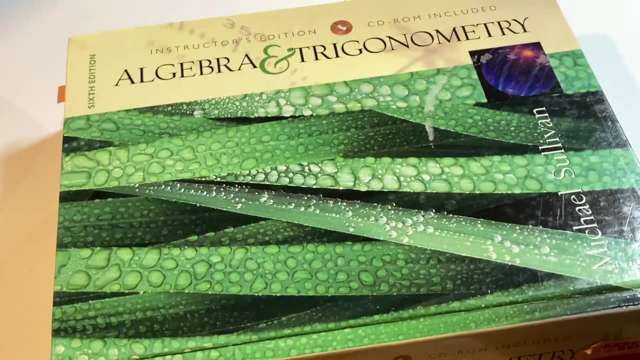 great book, um, excellent, just one of the best books out there. there's other good books. here's an example of another good book. so this book here is a book that i bought used and it's an instructor's edition of algebra and trigonometry by michael sullivan. 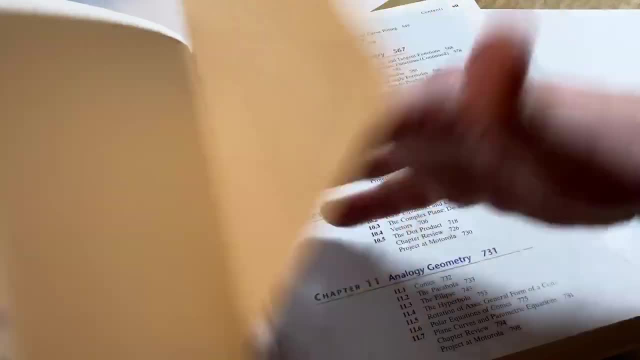 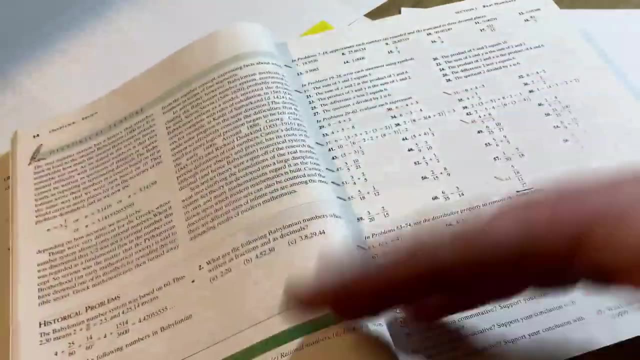 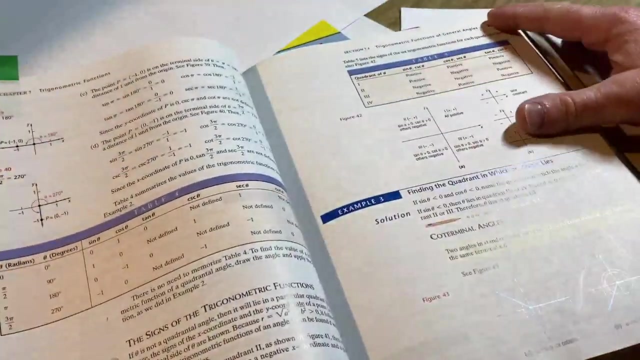 i got this used a long time ago on the internet somewhere and it has the same stuff that the book has. it just has different examples and slightly different exercises, so you get extra practice. i think it's nice having lots of books. as a person who collects math books, um, you know, i try to have you know at least one of every book if i can, but there's 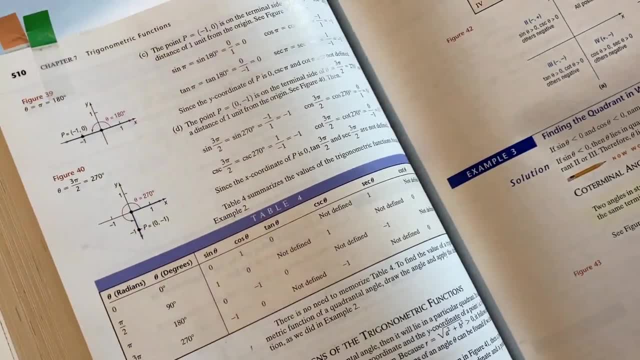 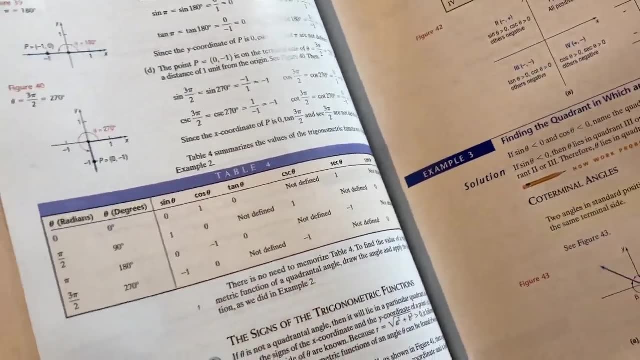 a lot of books that are really hard to find. this one is not right. none of these books are. all of these books are pretty easy to find. i'll leave you a link in the description in case you want to check them out. so the format's a little bit different. it's got like different tables different. 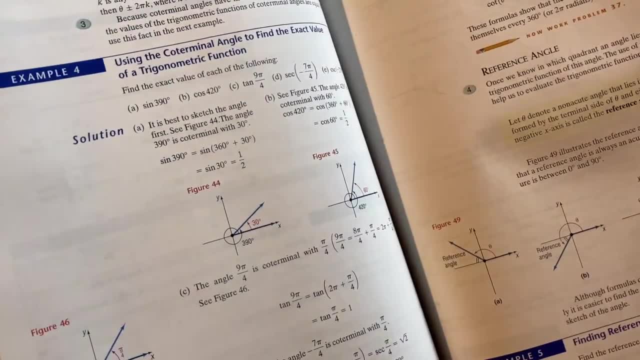 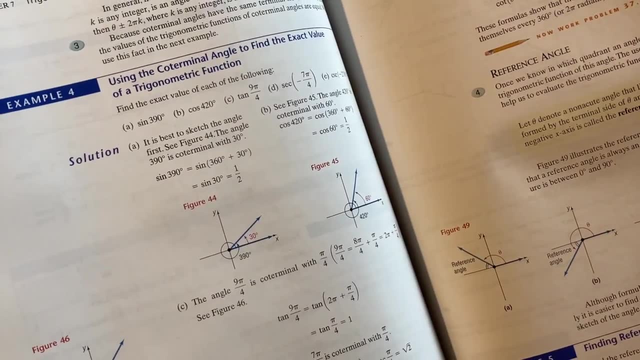 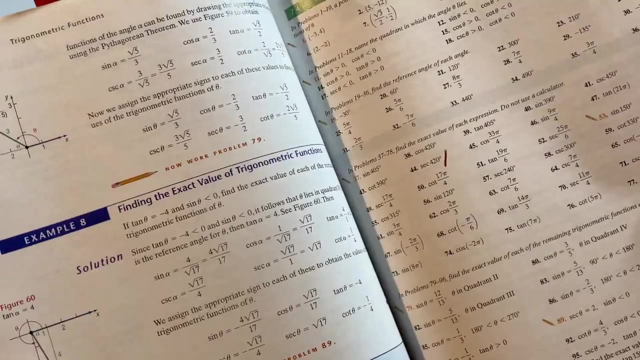 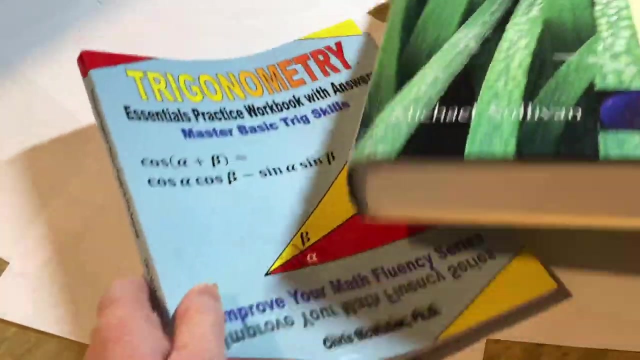 colors. but you see, he has solutions. find the exact value of your book and you can find the each of the following. so the sign of 390, cool, really cool, using some identities there. then you have some exercises here. so another great book for learning trig. and the last one is a book that 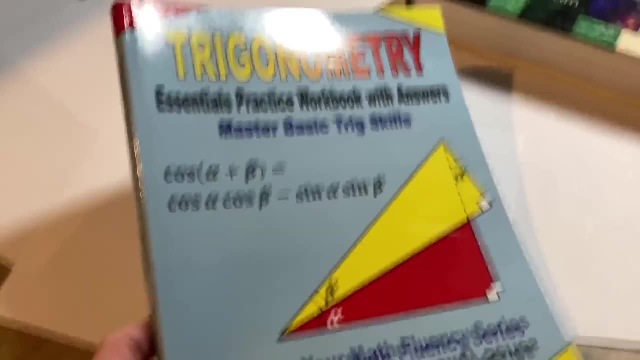 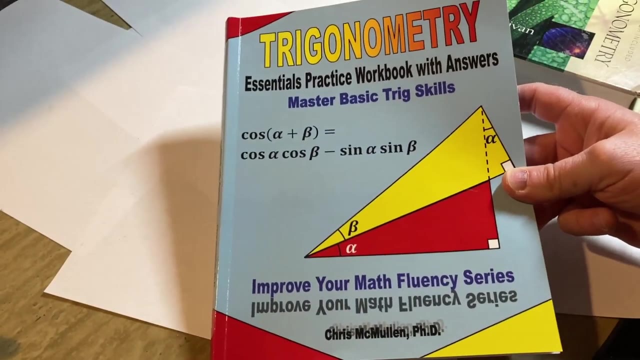 it's worth getting. it's the cheapest one of all of them and it's a relatively new book. it's called trigonometry essentials: practice workbook with answers- master basic trig skills. so this does teach you trig functions and he focuses on the important stuff, like the stuff you really need to know in order. 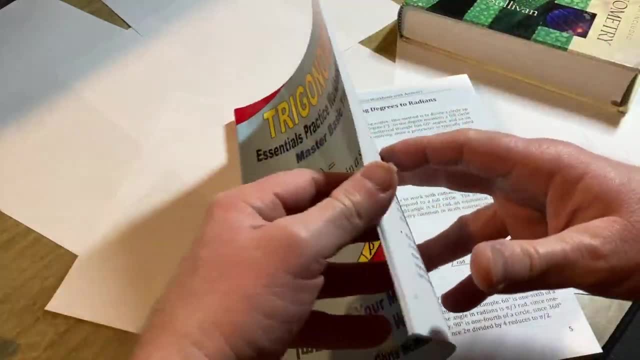 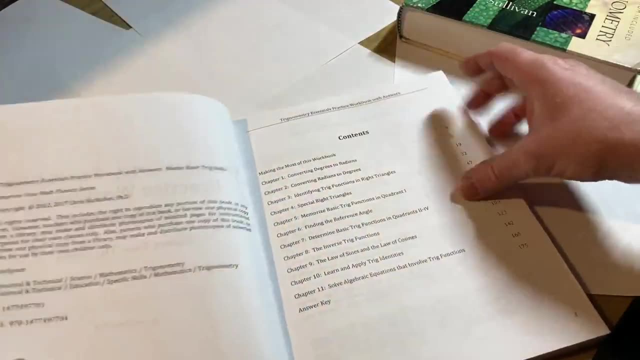 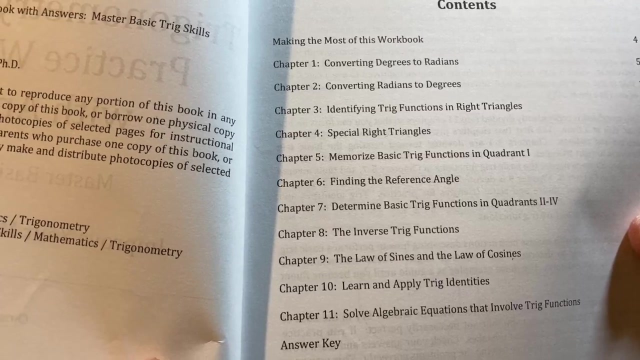 to, like you know, do well in the class and like pass tests, um. let me show you the topics because it's really interesting and he has answers to um everything, so everything has answers. so here's the topics in this book: converting degrees to radians. converting radians to degrees. identifying 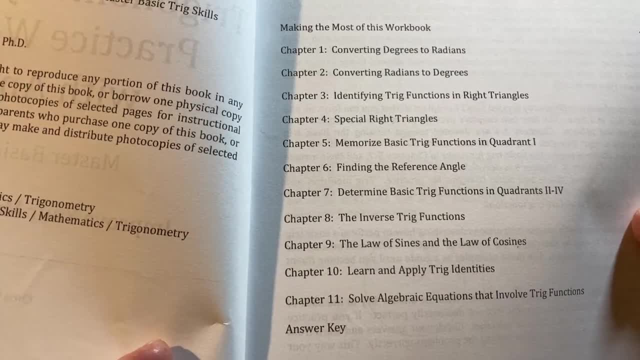 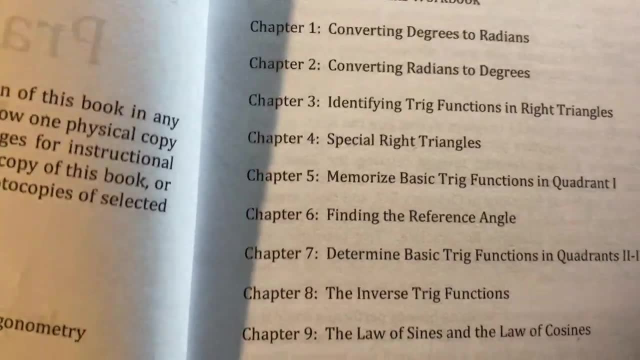 trig functions and right triangles, special right triangles. here we go. this is what i love about this chapter five: memorize basic trig functions and quadrant one. yes, yes, that is the most important thing, that's exactly how i do it. and then finding the reference angle and then determining basic trig functions and quadrants. 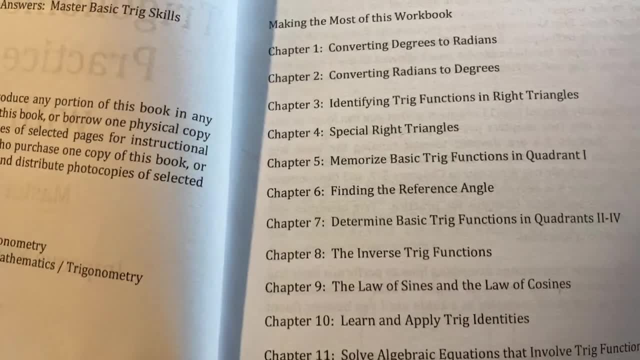 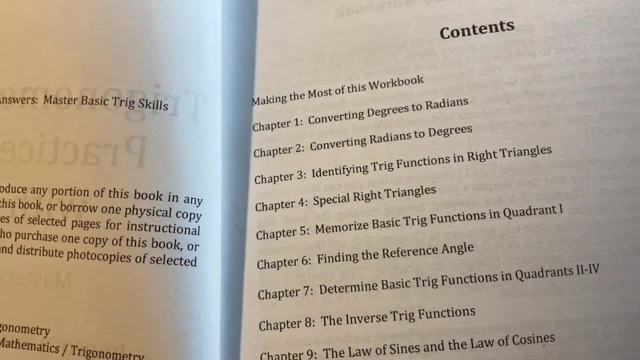 true to four. so right there, chapters five, six and seven, in my opinion, are the most important thing in this entire book, like if you're going to take away one piece of knowledge that's going to help you later, it's that. so you don't have to use your calculator or like simple. 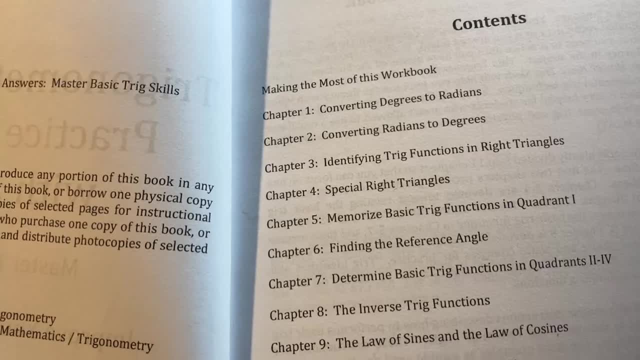 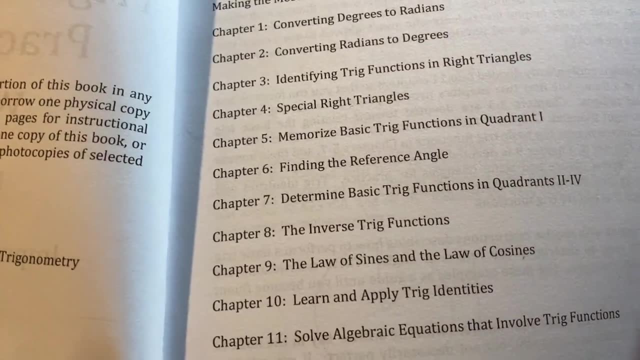 things. you can just look at it and say, oh yeah, that's you know, uh, that's going to be pi over 3 or to be, you know, the square root of three over two. so yeah, super useful inverse trig functions, law of sines and law of cosines: learn and apply trig identities and then solving some algebraic. 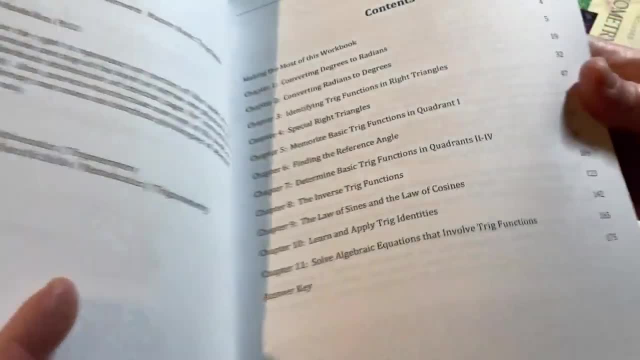 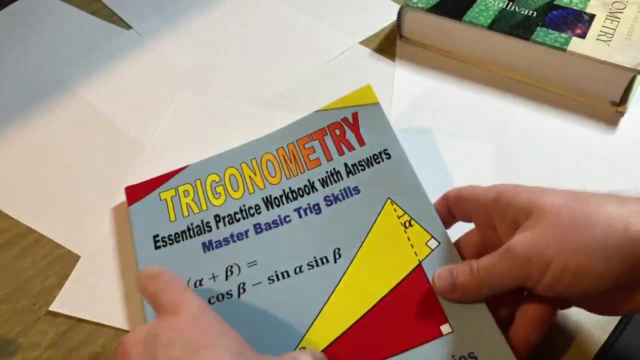 equations that involve trig functions and an answer key. he has answers to every single problem, not full solutions. he's really clever. so whenever he has solutions like, he'll put, he'll put solutions here, like if it says answers um, at least when i've checked, he just has the answers, but if he says you. 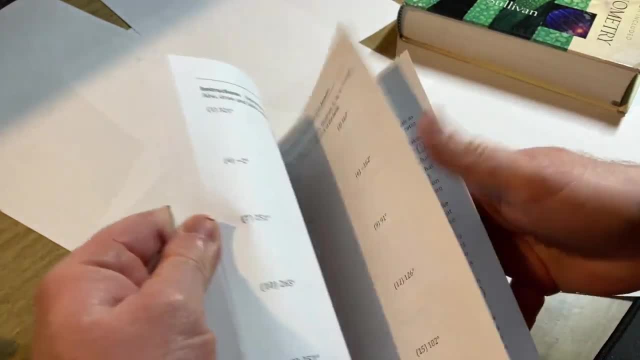 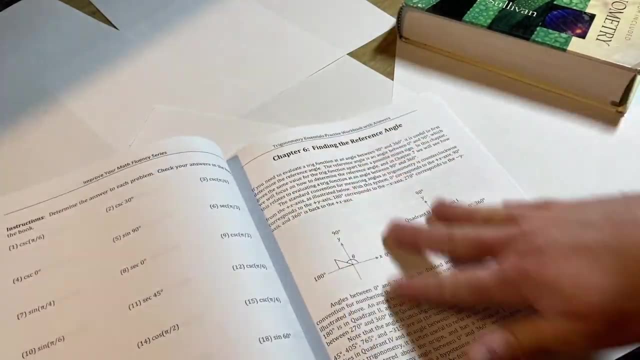 know full solutions. he's. he's got the full solution, so it's pretty cool. you can write in this book also. this is a workbook, so it's different from the other book. it's got tons of exercises and examples and it does teach you stuff, you see. he teaches you how to find the reference angle. he 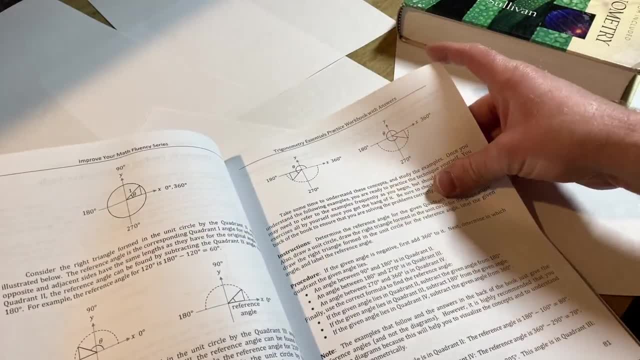 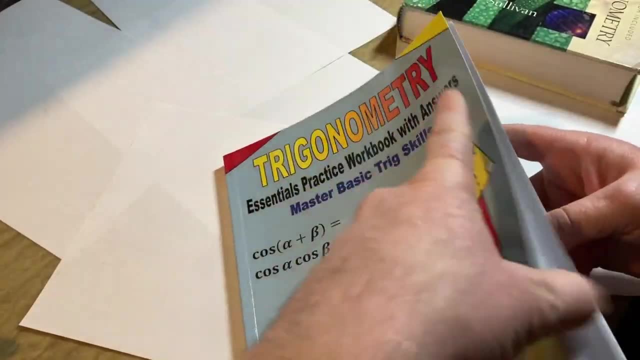 goes through it and then you know you do some examples and there's tons of examples, more than what you would find in a regular book on these particular subjects. so that's kind of interesting, so that. so that's something that you do get. i never really thought about it because you know. 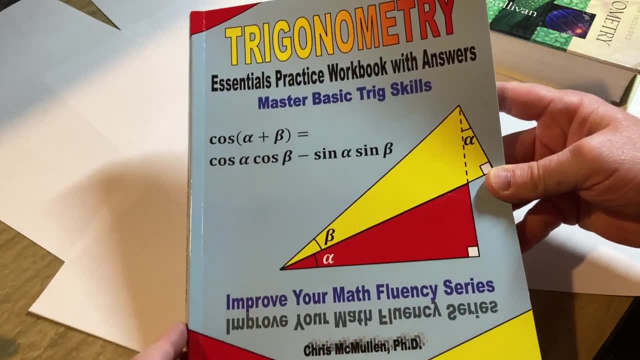 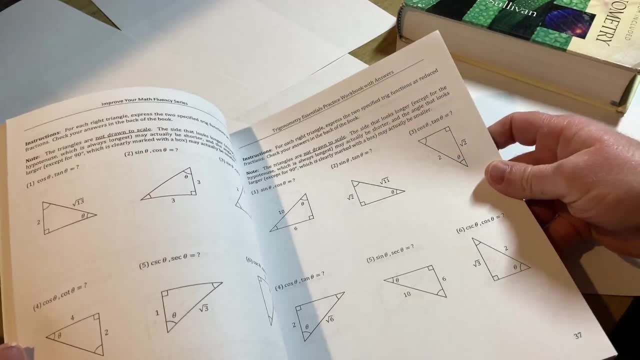 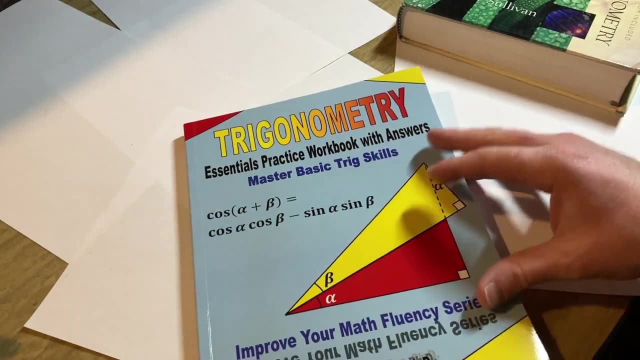 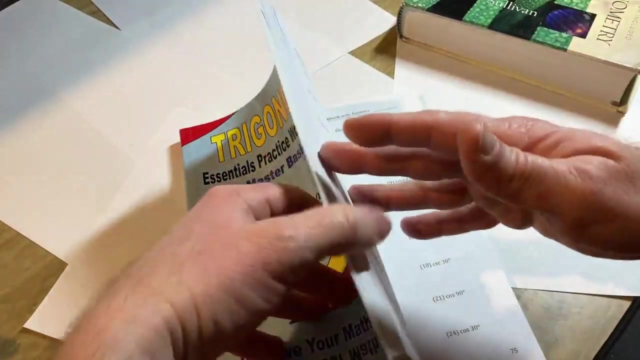 um, in many cases he has more examples than what you would find in a regular book on that specific topic. those other books i was showing you earlier- the sullivan book and the book by stewart- those books have more content, um, but, and they have more varied examples, right? so i mean, that's just a lot. 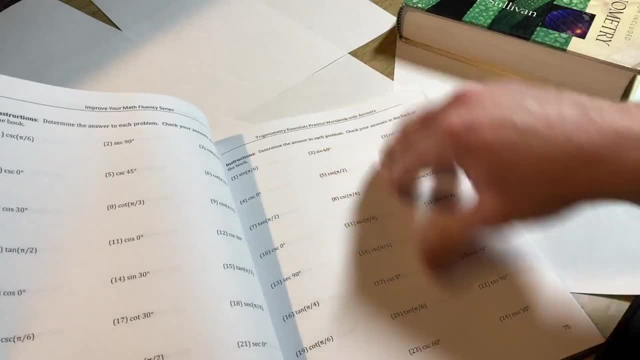 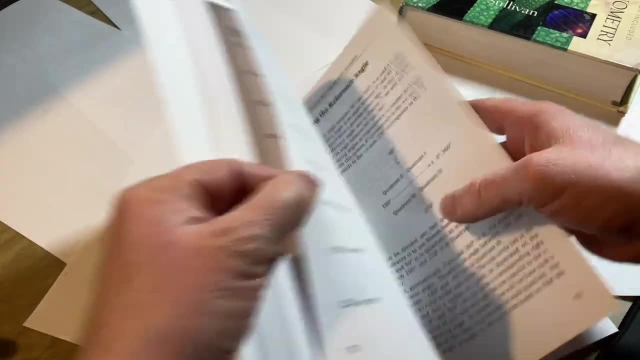 right, look at that. it's just a lot of examples. one through 24. let's turn the page. oh, look again. one through 24, again i mean, look at that. and then one through 24, again i mean, it's just so many. one through 24.